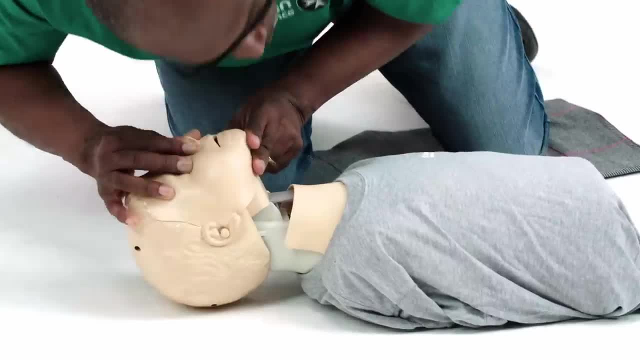 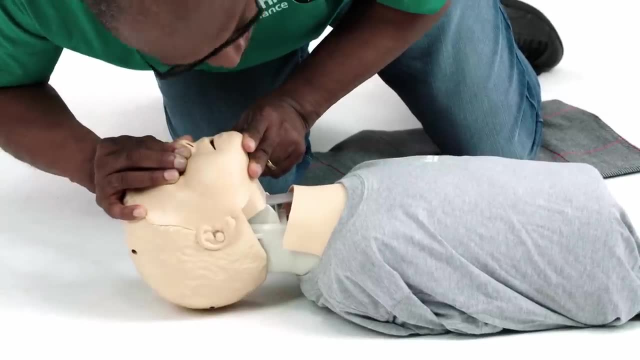 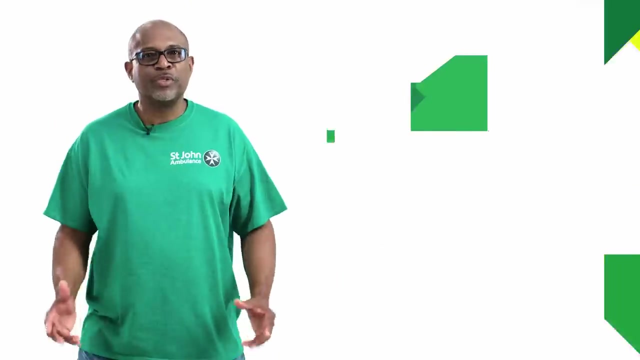 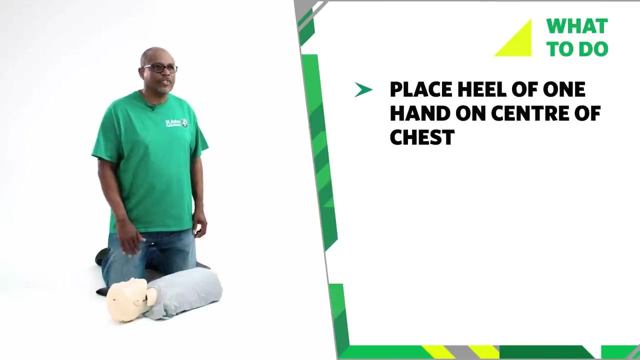 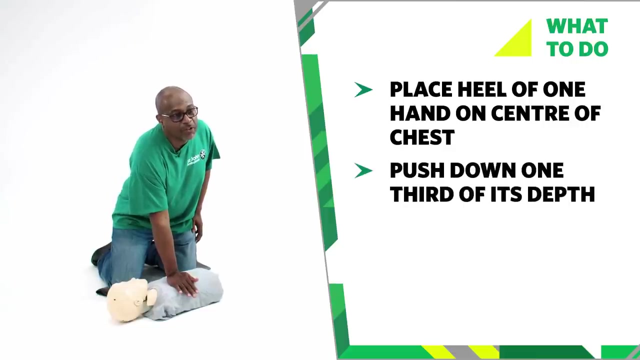 this To do chest compressions. kneel down by the child beside their chest. Place only one hand on the center of the chest. Lean over the child with your arms straight and press down vertically one third of its depth. Release the pressure. Allow the chest to come back up without removing your hand from the 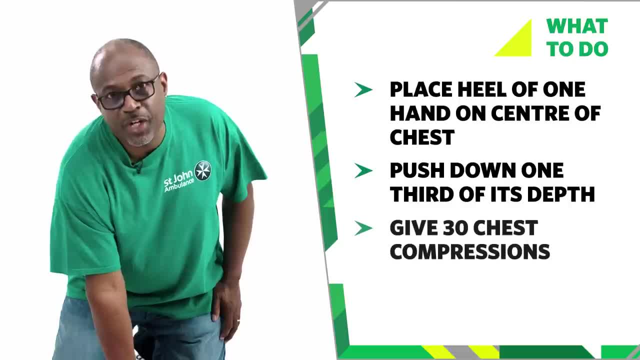 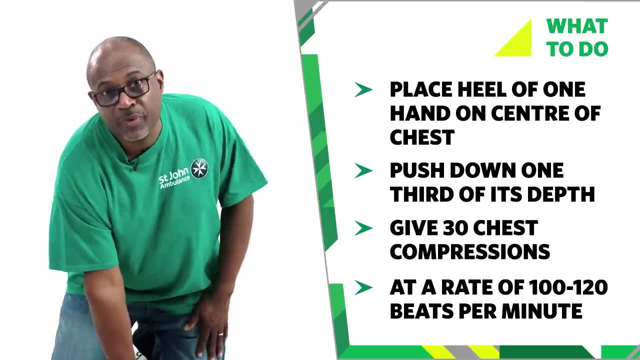 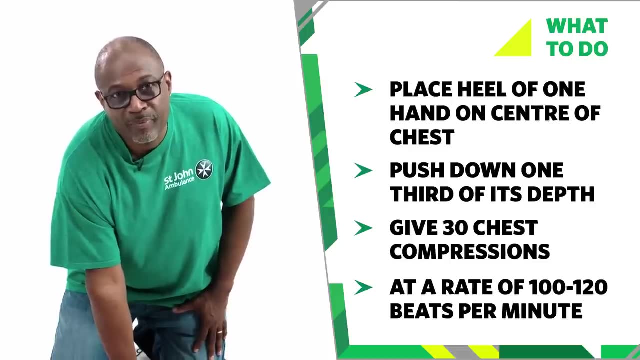 chest. Repeat this to give 30 chest compressions at a rate of 100 to 120 beats per minute. This is quite fast and to help you, you can sing Nelly the Elephant, which can help you to keep up with the pace. 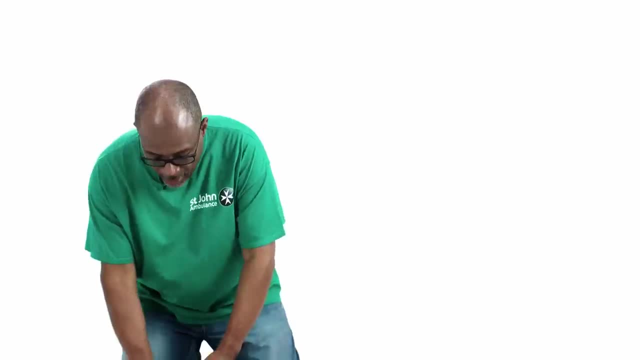 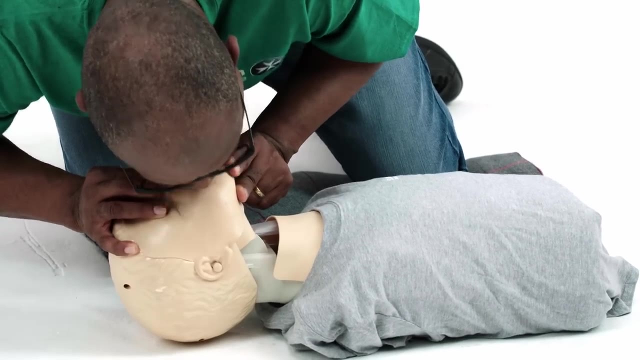 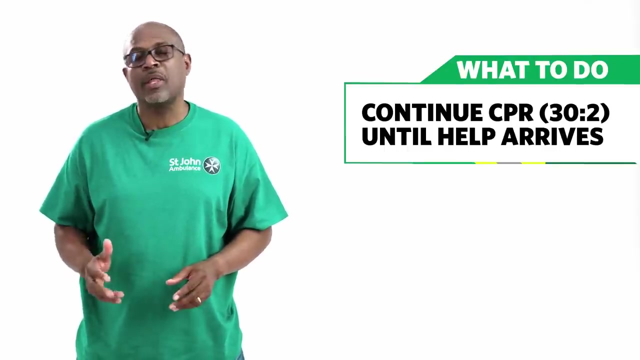 After 30 chest compressions, open the airway and give them a further two rescue breaths. Continue to alternate between 30 chest compressions and two rescue breaths until help arrives. If you are on your on your own and don't have a speakerphone, stop after 1 minute and 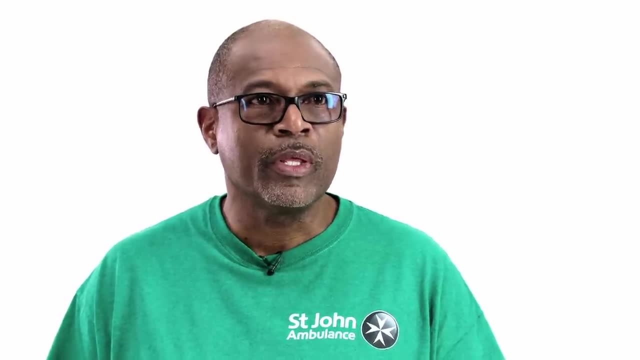 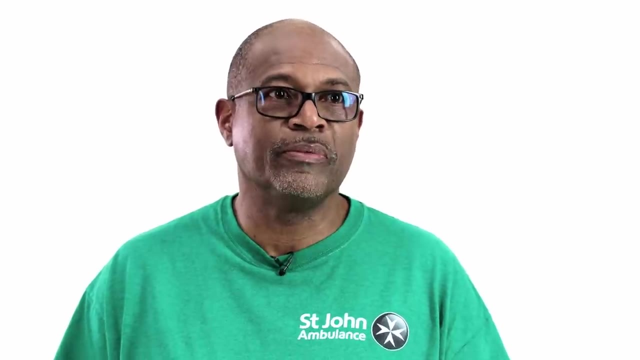 call 999 or 112 for emergency help. If your mobile phone is not available, contact the and you have to move to get a telephone. take the child with you if you are able. Do not leave the child to look for an AED. The emergency services will bring one with them. 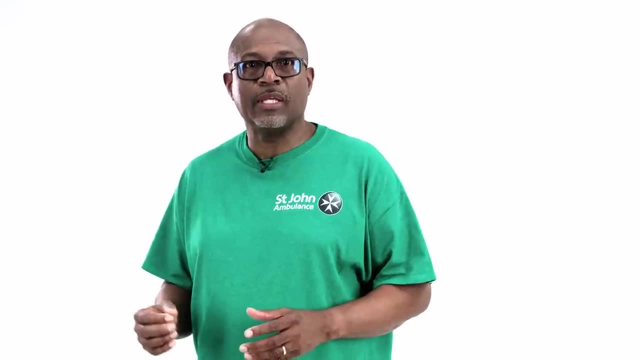 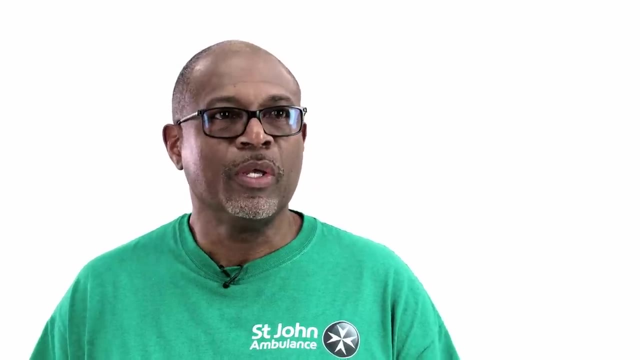 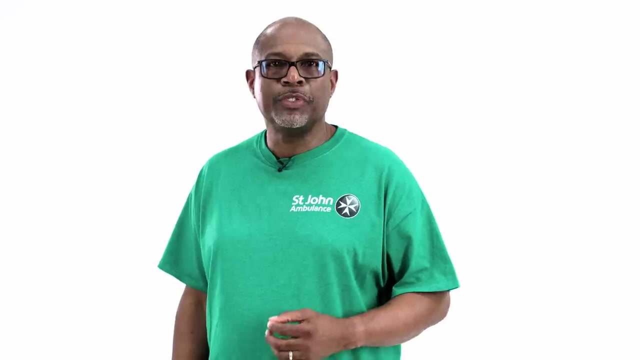 If there is someone there who can help. if they have brought an AED, ask them to turn it on and follow instructions while you continue CPR. If they can help you perform CPR, you can swap over every one to two minutes with minimal interruptions to chest compressions. Continue CPR until emergency. 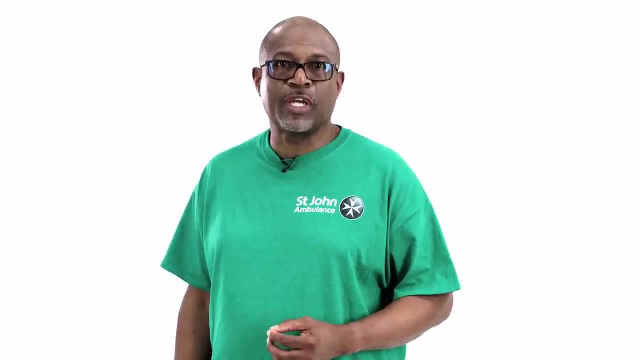 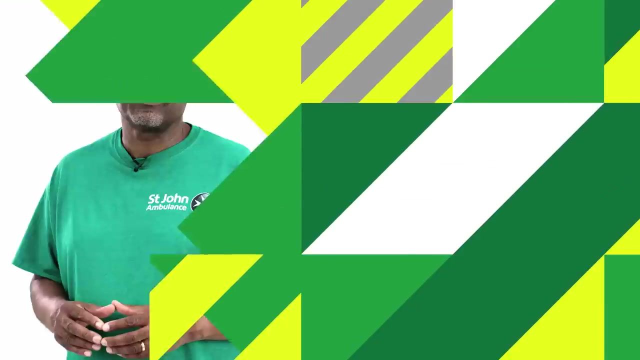 help arrives and takes over, the child starts to show signs of becoming responsive. they start breathing normally or opening their eyes, or you become too exhausted to continue. If they do start breathing normally, again put them in the recovery position. So remember, if you come across a child, that's unresponsive.